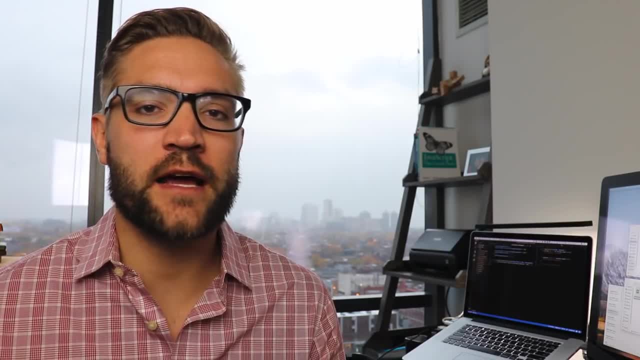 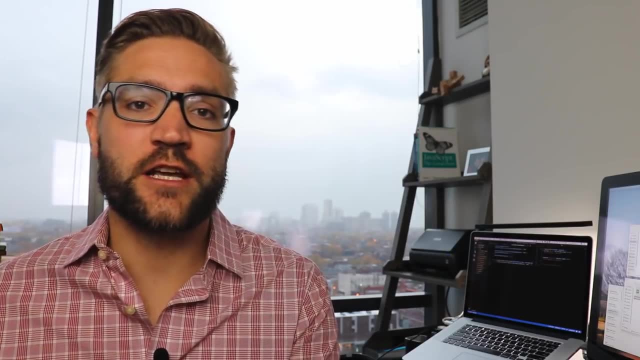 or what you may call manual testing. So they're assigned to change or add some business logic to the application they're working on. right, So they will go into the code, make some changes and then the way that they'll test their code to see that it's doing what they want it to do is they'll go into 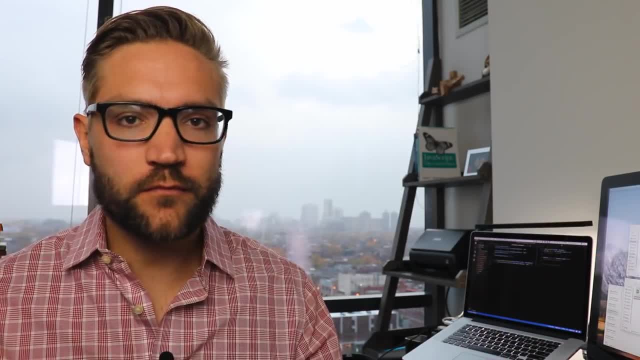 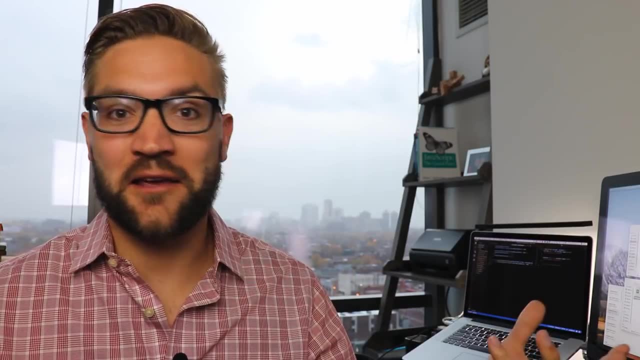 the browser, they'll pull up the application, they'll hit the refresh button and they'll look at a certain piece of data that they know should be coming out a certain way, and if it's working, then they okay. they've done their job, But manual testing. 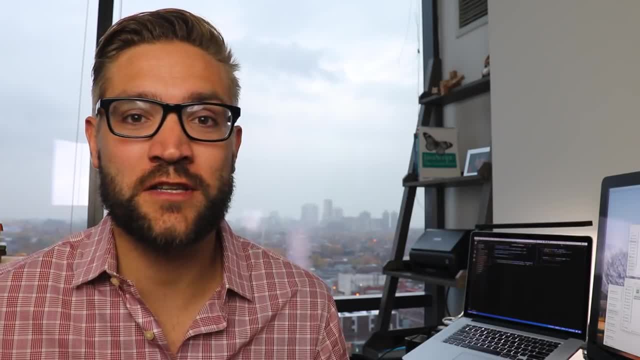 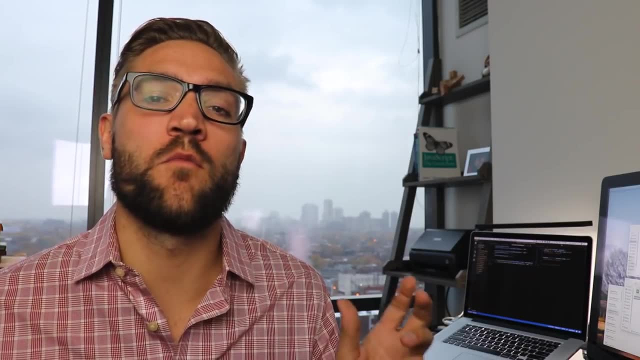 has its limitations and if you're building a large application that is constantly adding complexity, not having automated tests in general but, even more specifically, unit tests that you know test the fine-grained logic of the smallest components of an application. 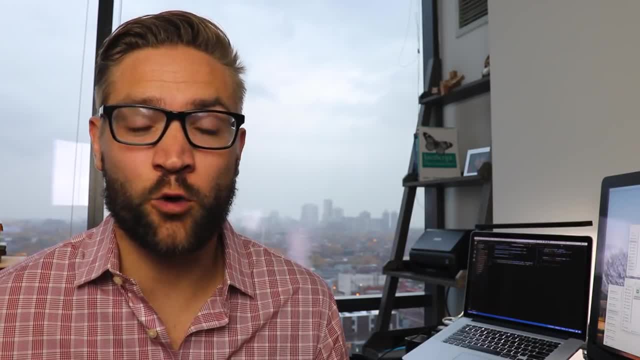 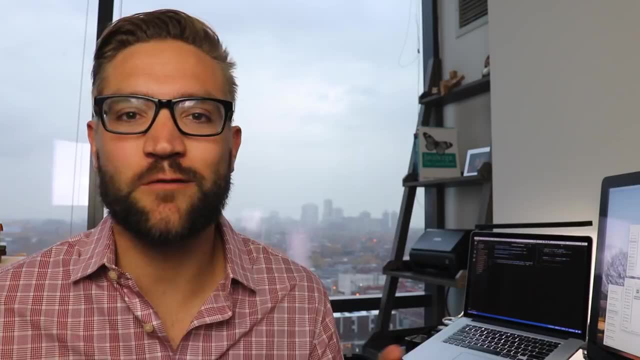 are going to. it's just going to be tough to maintain a working application that doesn't have a really high bug rate, So we'll dive into unit testing- exactly what that is. So you may have heard unit testing and many people will say unit tests, when they actually 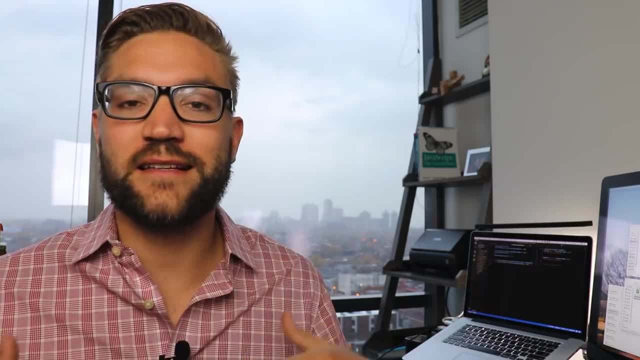 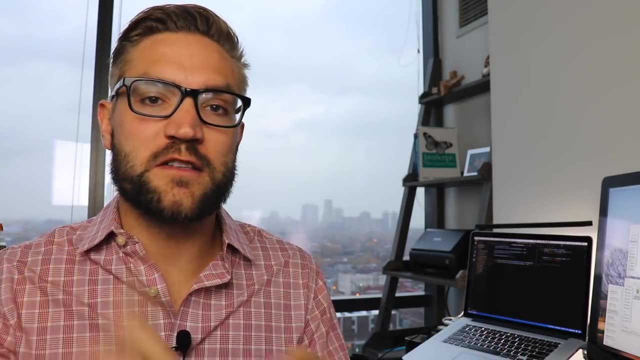 are talking about just automated tests in general, And automated tests are basically tests that run automatically or are programmatically run. that can test a wide range of things. So a lot of times you'll hear about smoke tests. so typically that is front-end. 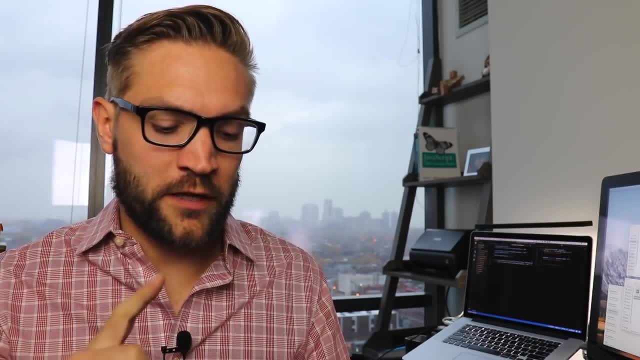 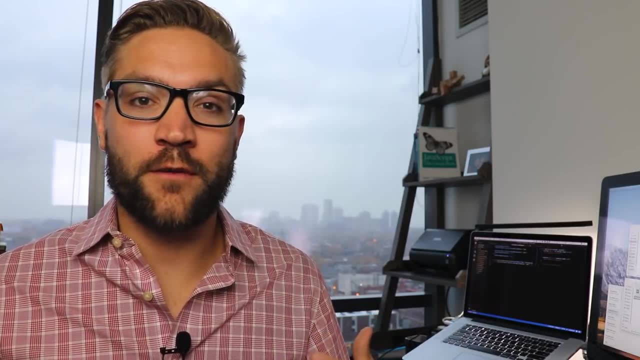 testing or the user interface testing. You can hear about acceptance tests, which are typically testing endpoints to make sure that the model that's being returned from endpoints are correct. There's also integration testing, which is testing that the application or any external integration is working. So you can see that the application is working and you can see that the 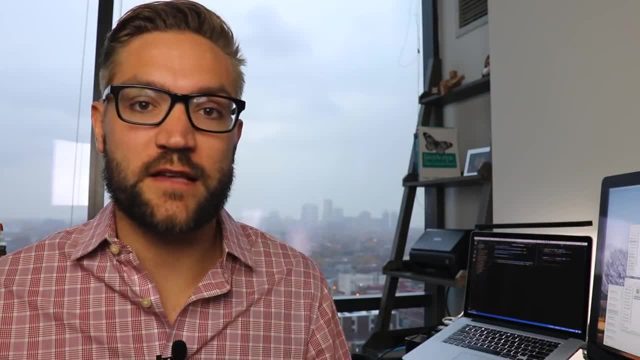 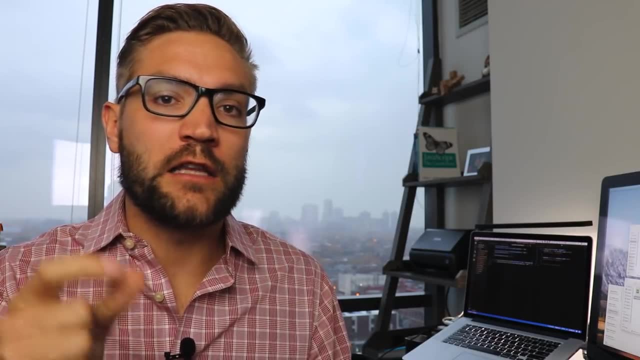 operations of that application are working as expected. And then there's unit testing, or I call it in-memory testing. that tests the smallest components of the application and their fine-grained logic, or business logic. Now, in order to unit test your application, you have to follow the 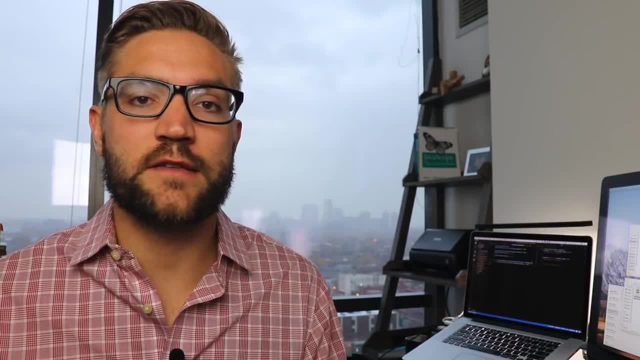 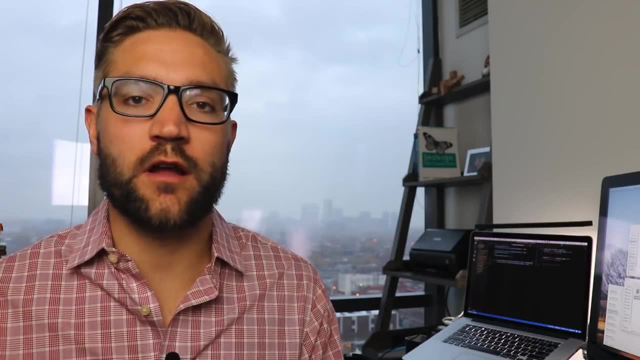 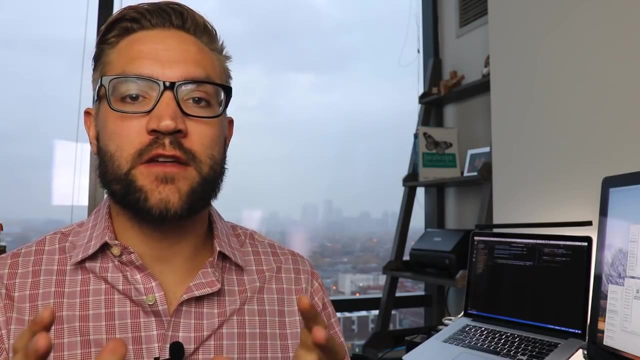 design principle of having small modular components that you can test. Now, the reason that I call unit testing, in-memory testing, is because if you're going to test a small component of an application, it cannot be connecting to the database, it cannot be connecting to an external integration. it is meant to do, it is meant to be encapsulated. 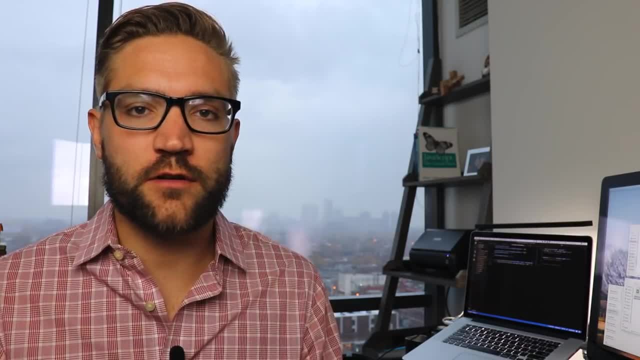 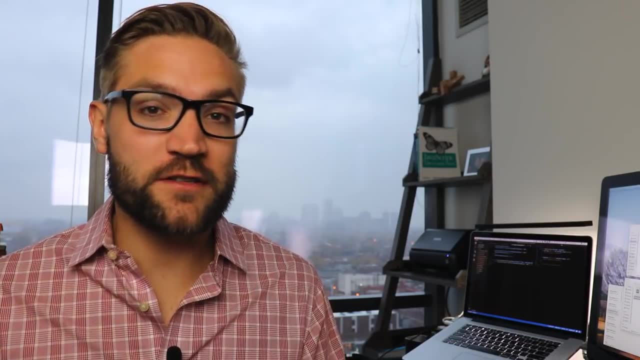 in-memory. So you have to have an application that's structured of small little modular components that, for example, if it does connect to a database, it can be mocked. You'll hear a lot of references to mocking when you're doing unit testing, because you want to make sure that any 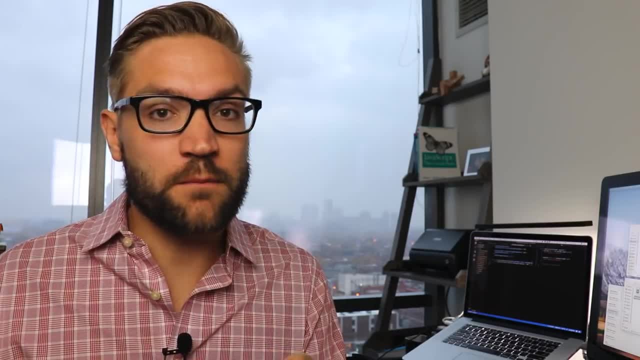 external dependencies. so any components that rely on another component to do something need to be. they need to be faked, they need to be stubbed, they need to be mocked. which is basically saying, like you're creating a new component, you're creating a new component, you're. 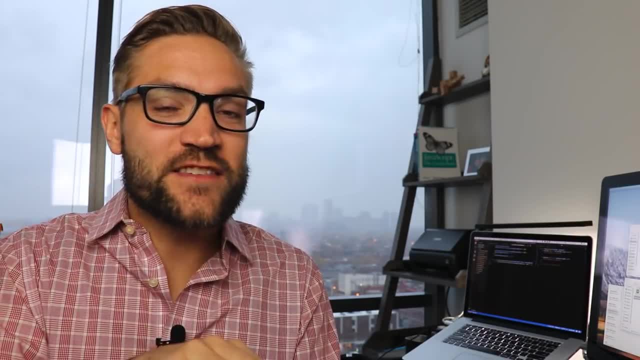 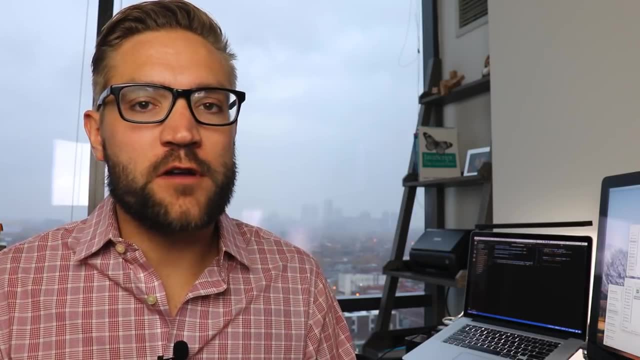 creating a fake implementation of that functionality and you're inserting it into the component that you're testing, so it doesn't actually, for example, call the database. This may be something that you'll come to understand over time. you don't necessarily have to understand. 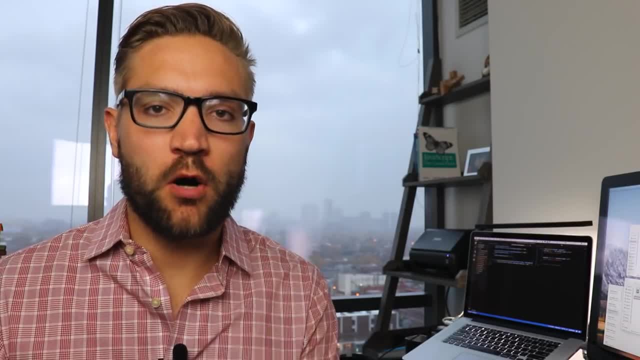 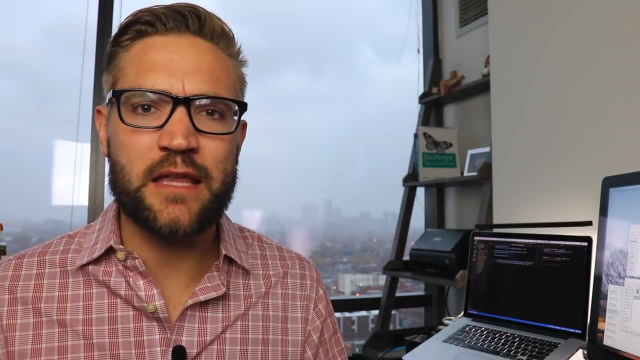 it now. So, going on this idea of having small components in your application, it's good to remember that each one of these components needs to do one thing, and do it very well. A good example of this may be like an email service or an email component that simply has one method on it, or 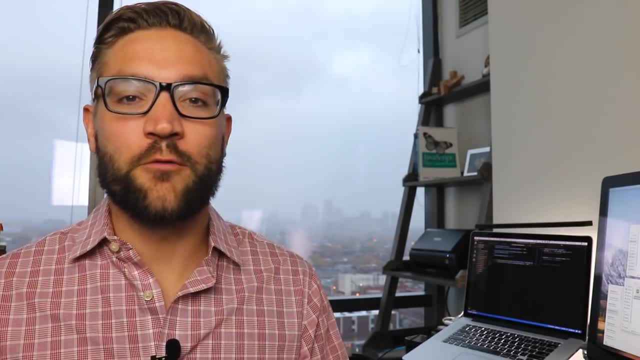 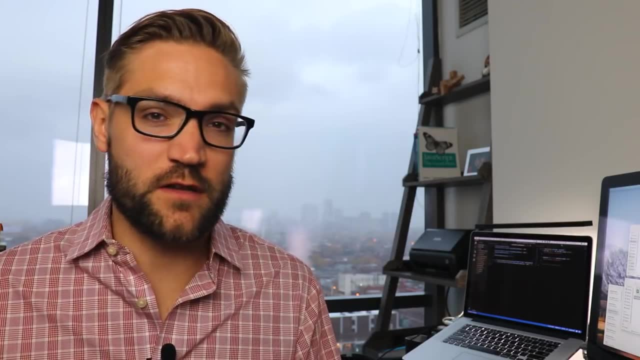 maybe two methods And that just emails or sends out emails. The reason that you wanted to do one thing and one thing only from a unit testing perspective, is you want to test the logic of the email service and the email service alone. So if the email service is sending out an email, sending notifications to, 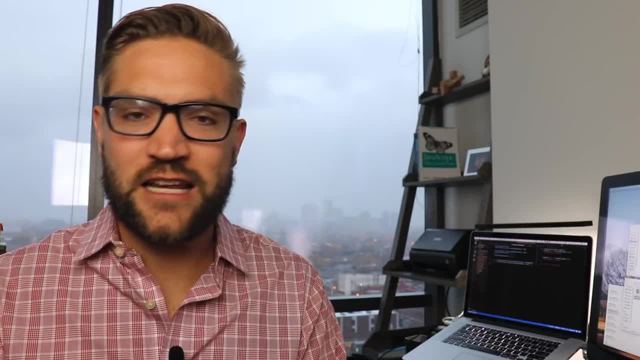 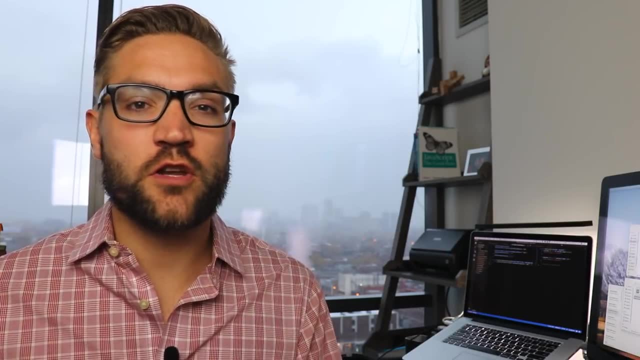 the user interface if it's reloading or refreshing the database. for some reason, these are all separate actions and really any component should just be doing one thing, So you shouldn't have to test everything that's being done. Okay, so now that we've covered unit testing, we've 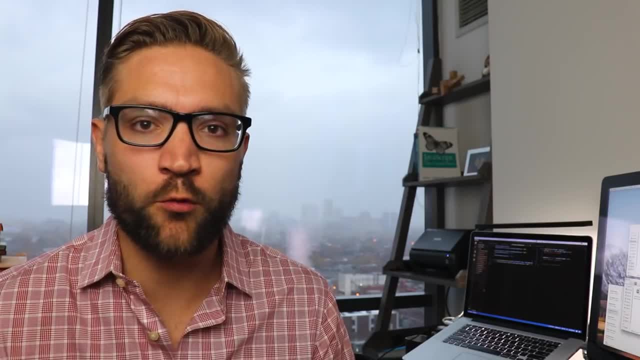 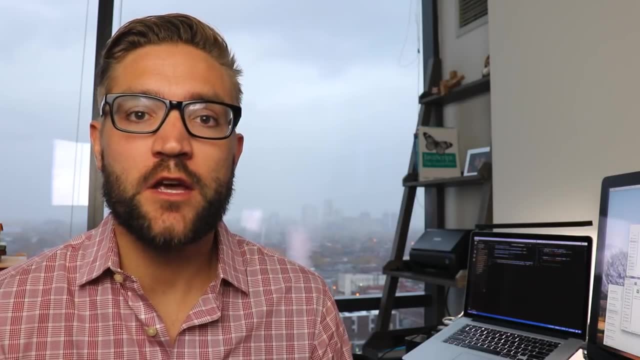 got to explain how, in order to really truly unit test the correct way you need to do in memory testing, And that requires that you have small testable components. So I'm just going to do a dead simple example. I'm going to use C sharp. if you don't know C sharp, this still should be somewhat. 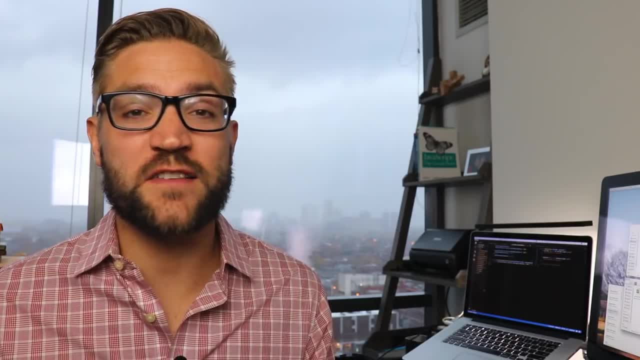 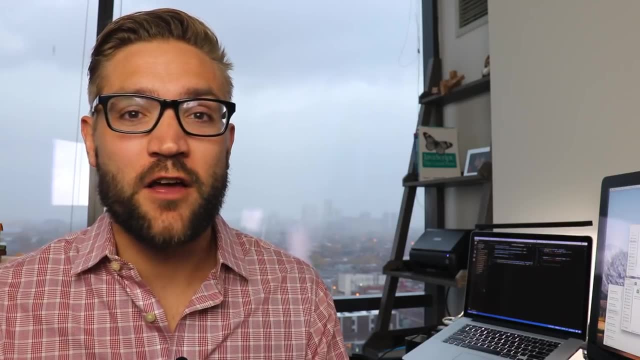 readable to you. I'll include this application in a GitHub repository, So check the link in the description below if you want to go ahead and download that locally. But other than that, it's pretty simple. I'm just going to have really two main components of the application, So I'm going to 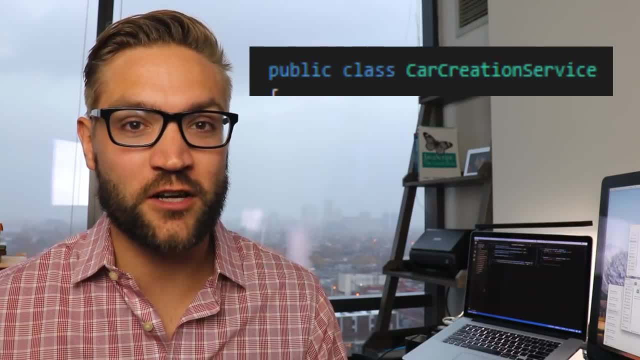 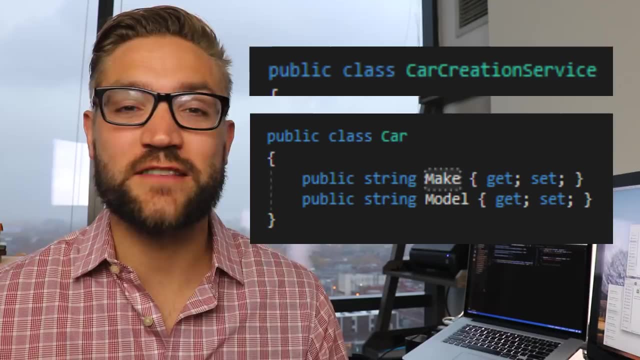 have a car creation service that's going to create two different types of cars. it's going to have two methods in it And then you're going to have a car class which just has two properties: a make and a model property, both which are strings. Now let's go and take a look here at the car creation. 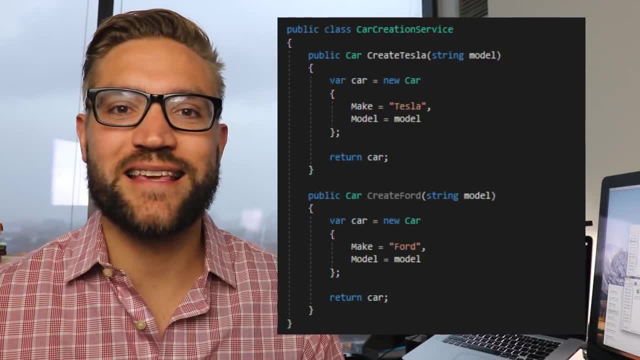 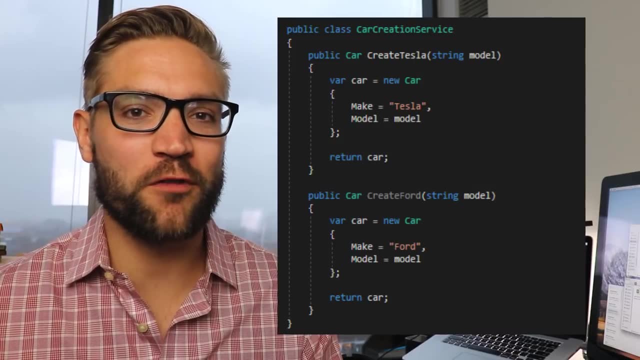 service. The two methods on there both accept the same argument. you're going to accept a model which is a string, and it's going to assign that to the car that it's going to create And, as you can see, both methods are named for the type of car that you're going to be using, And then you're. 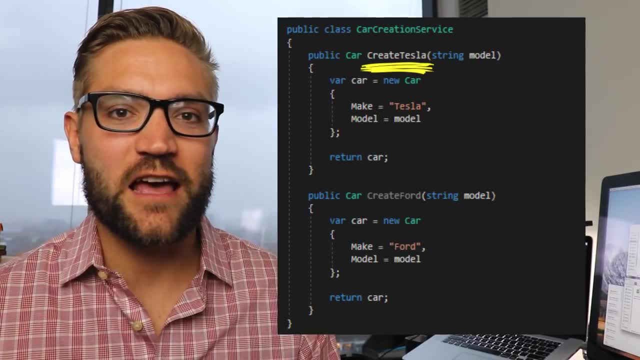 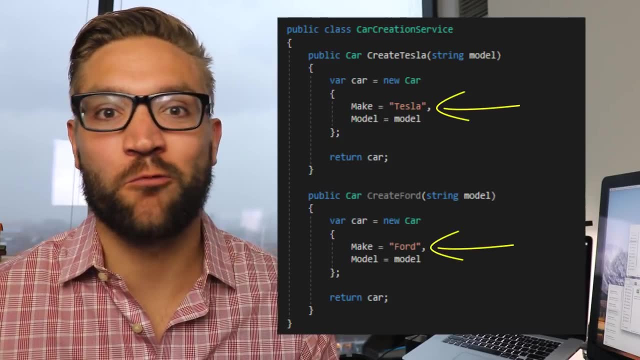 going to have a car that they will make. So one's going to create a Tesla, right, And the other is going to create a Ford And you can see in the make properties being set in each one of these methods based on what type of you know what method you're calling right. So it's going to create a 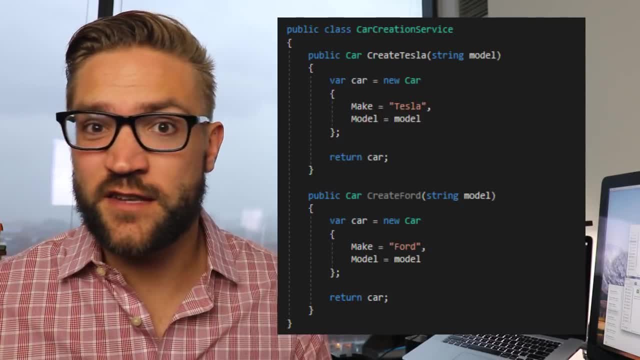 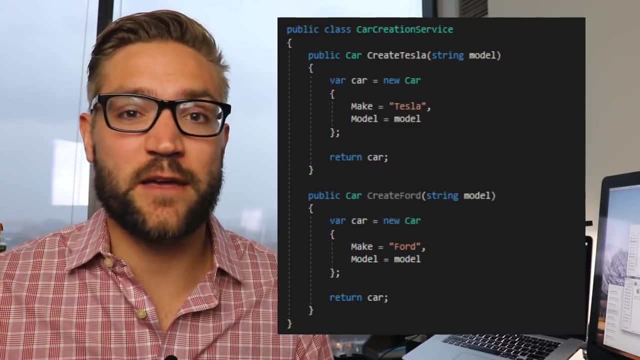 Tesla is going to create a Ford. This is very easy As you can see. it's a creation service. it's creating a car object or car class, And that's going to be very easy to test. So let's actually run to what a test may look like for this. So I'm going to drop down the creation. 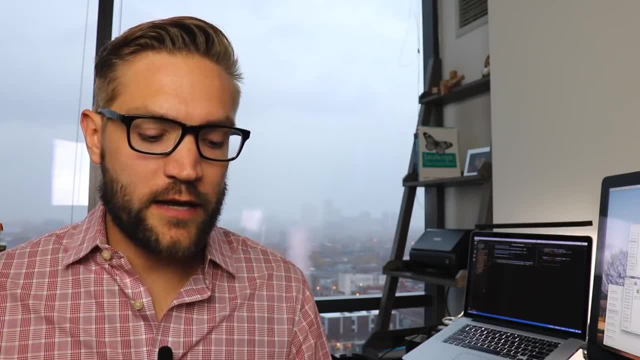 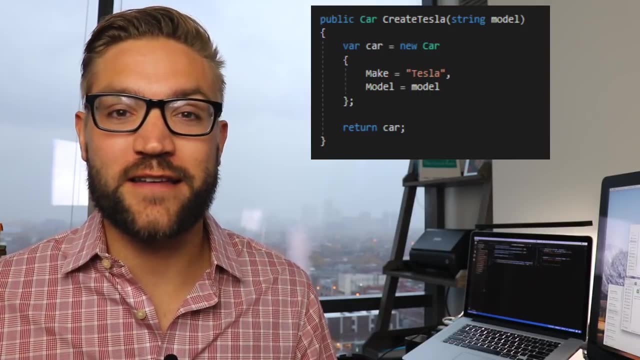 service. we kind of have a good sense of what that is, But let's go ahead and test that. Let's go ahead and test the Tesla method. Now we really have two pieces of logic in here that we need to test. we need to test that the make is set correctly and the 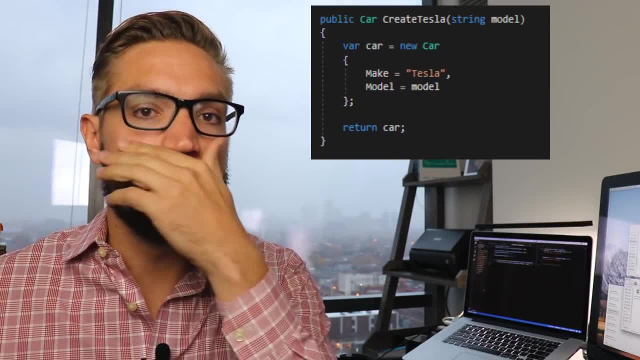 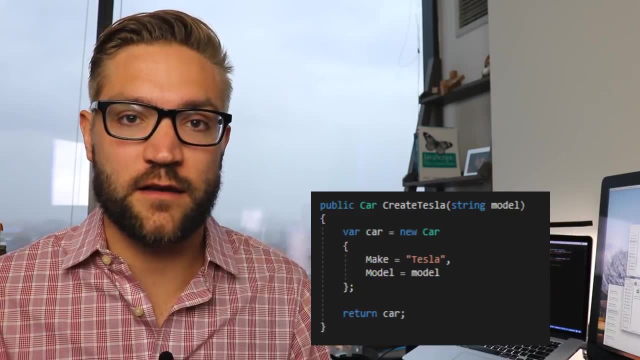 model is set correctly. So I can really consider that two separate tests. So first let's go ahead and write a task for ensuring that the make is correct when we call the create Tesla function. So we're going to create a test here. At the very top you'll see a test attribute that tells our 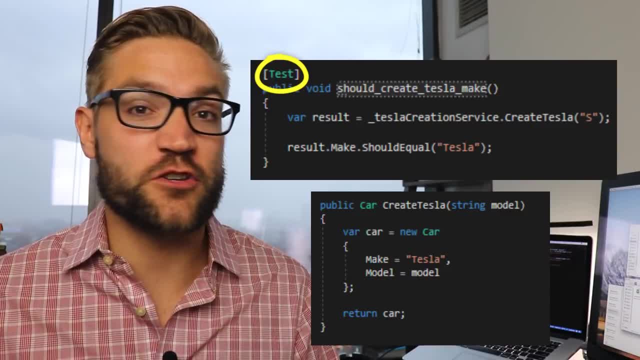 our testing framework that this method that we've written is a test and should run it as a test. So we're going to run it as a test. And we're going to run it as a test. And we're going to run it as a test, Then we name that method aptly so that you can tell what should be what. 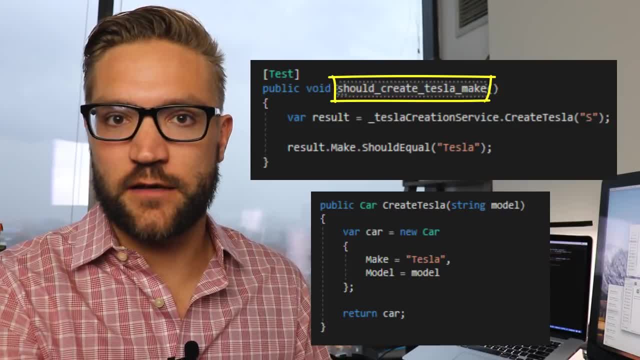 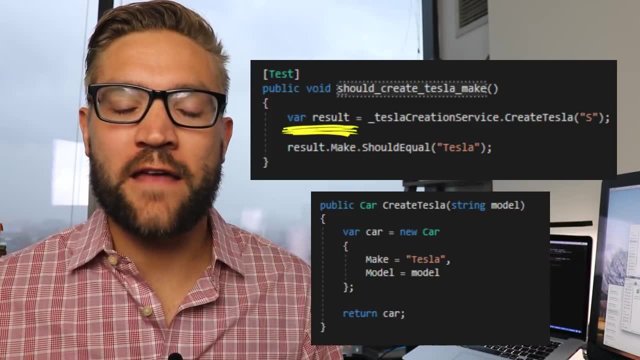 the outcome should be right. So I'm saying should create a Tesla. And then what we're doing inside of here is we're we're calling that creation service, we're storing that in a result variable And then we're saying that result should equal Tesla, should equal the string Tesla. Now, if we 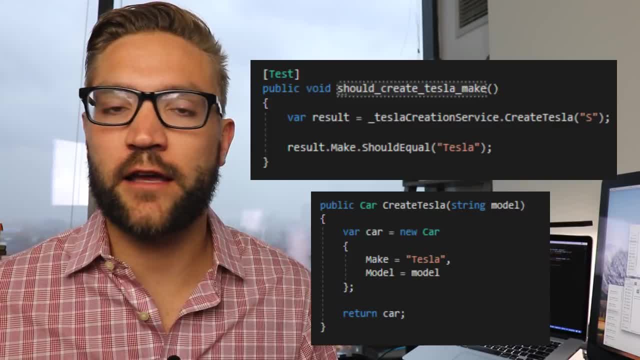 run this right, so I have using re sharper as a test runner. if I click the run test button here, the test result will come up. pretty much as we expected, I'm expecting to call the create Tesla method. that will create the result, And then we're going to call the test result And then we're 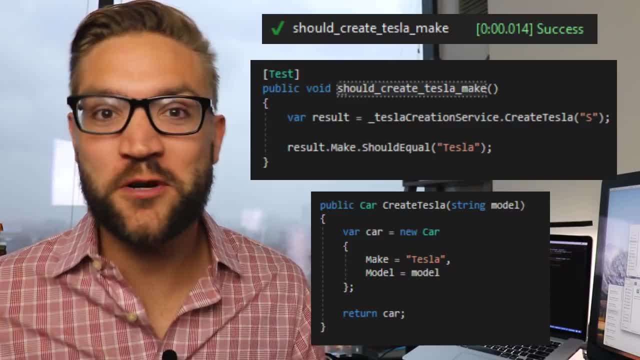 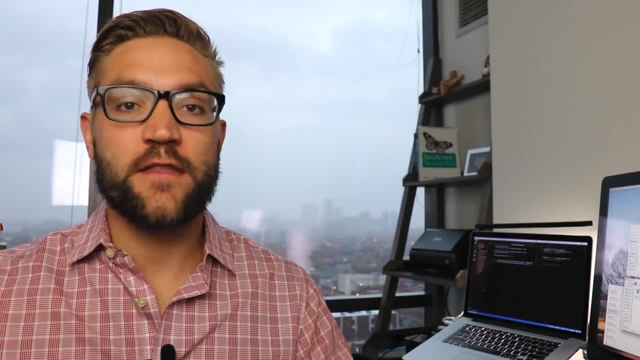 going to create a car that has the make- Tesla. that is pretty easy, pretty dang simple, to understand. The key thing here is that we're testing different pieces of logic, So let's move on to the next piece of logic. So the next piece of logic that we want to test. 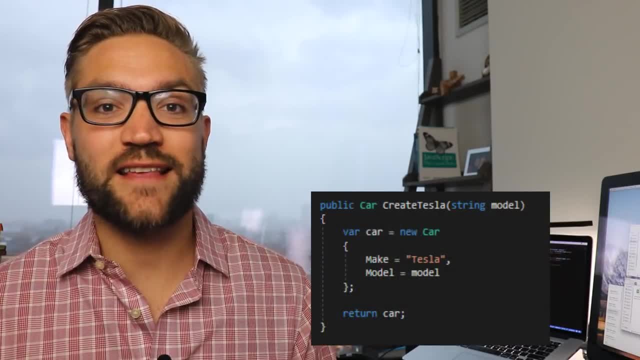 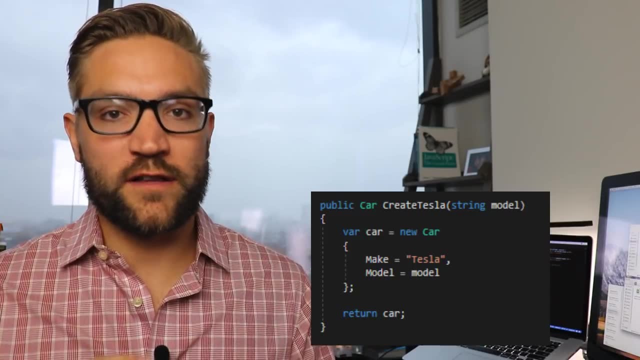 and I'll go ahead and throw up the creation service Again, just to give you a sense. here we want to test that the argument we're passing in is being set on the car object or car class. So let's go back to the test here And we're going to create a brand new test And, as you can see, 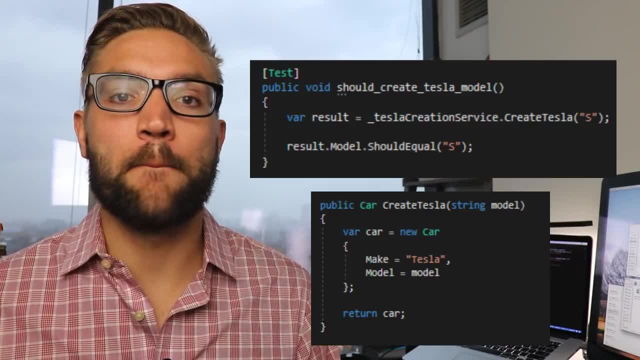 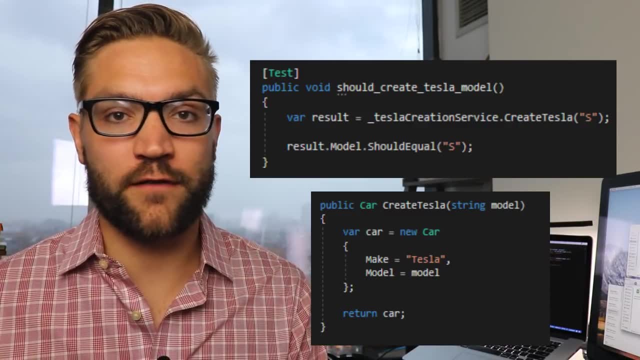 all, everything's pretty much the same. we're going to be asserting that the model is as we set it. So in this case I'm setting it to be the model S. I want to make sure that the result of the resulting car that's created will be set to the correct model. So if 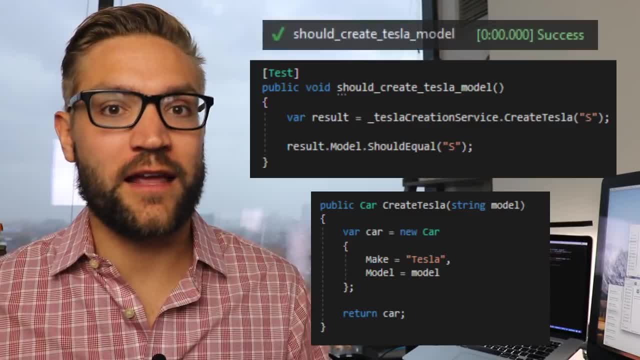 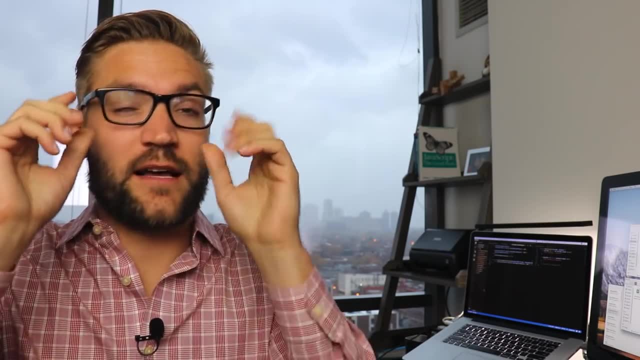 we run this test based on everything so far. this should work And it does right. So it's telling us everything passes, everything looks good. Let's say: come back to this code later. And I'm really tired And I'm, you know, my glasses are a little bit crooked right, I'm working on the code And 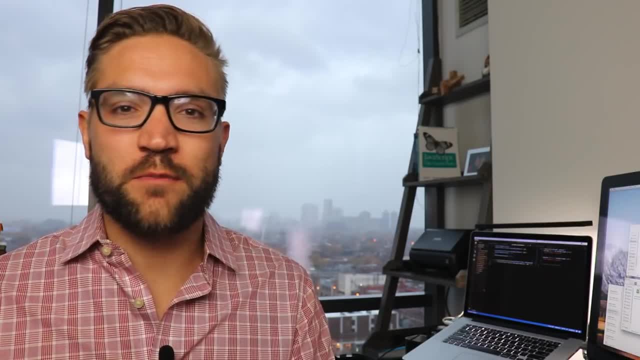 I'm working on the Tesla method, Say. I go in there and I didn't see what I was doing, But it's like: oh, this is the Ford method And I just changed that to Ford, So let's go ahead and see what that. 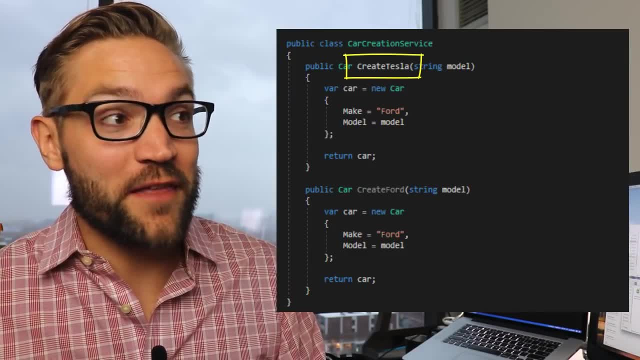 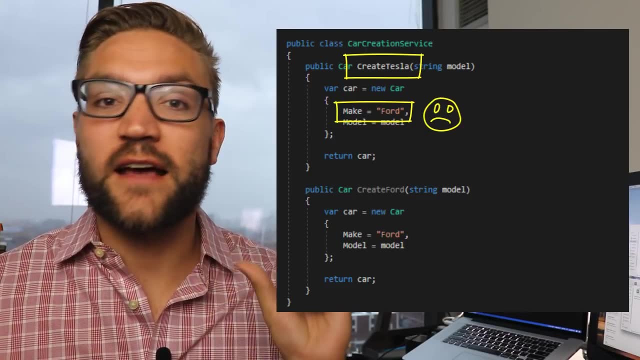 would look like. Obviously it's not correct. We see it's the Tesla method, but yet it's setting it to Ford, So this should break our test right? This should be if, assuming that automated tests are run all the time, it's going to run this unit test. if we go ahead and run it, what's really? 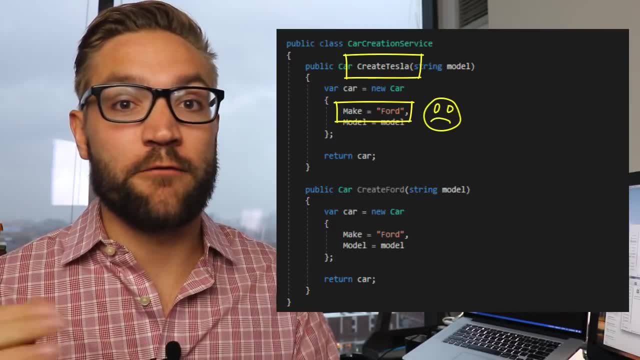 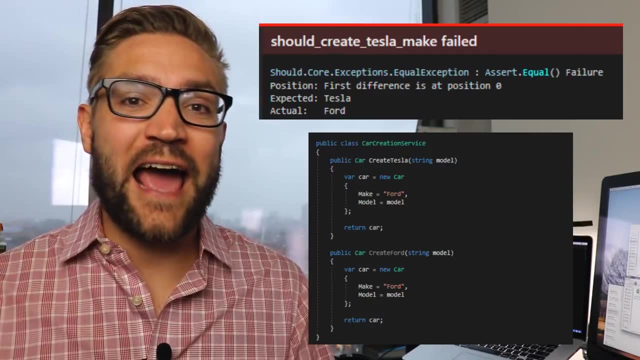 nice about n unit and our re sharper test runner is that if we run it as you can see here, it gives us a very clear indication of what the expected result is, what the actual output is, and so I'm given that instant feedback. So if I'm really tired, I run those tests. I go. 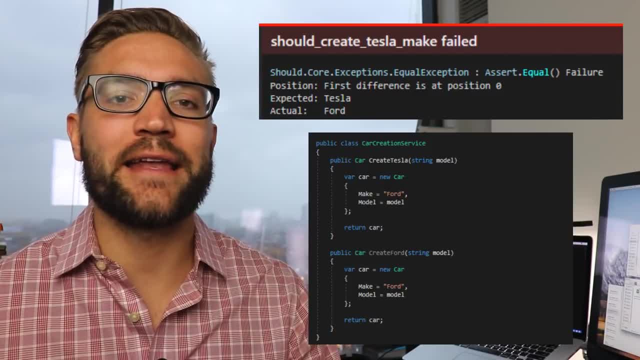 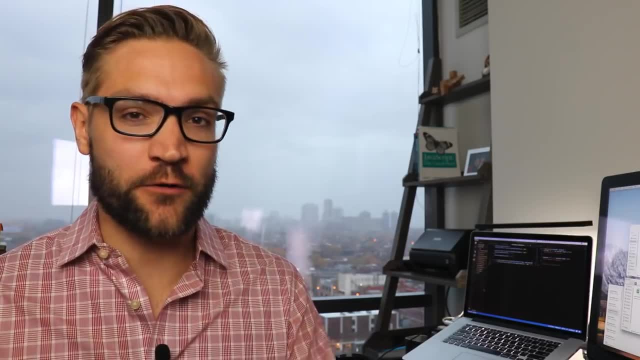 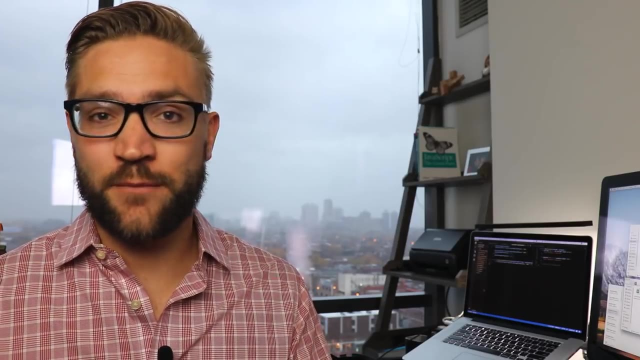 what the heck that a Tesla methods returning Ford. I can go ahead and change it, And what is really cool is that a lot of organizations actually will have some sort of continuous integration process that runs a task to run all of their automated tests anytime that a developer makes a commit. 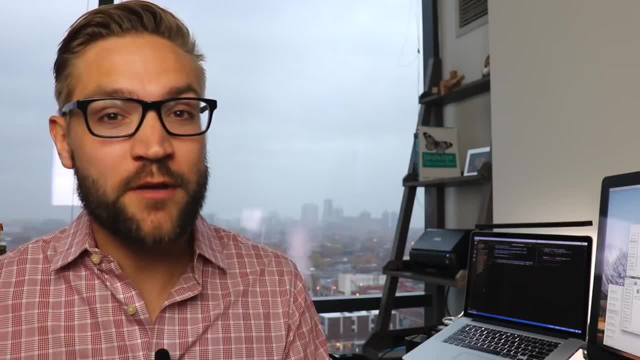 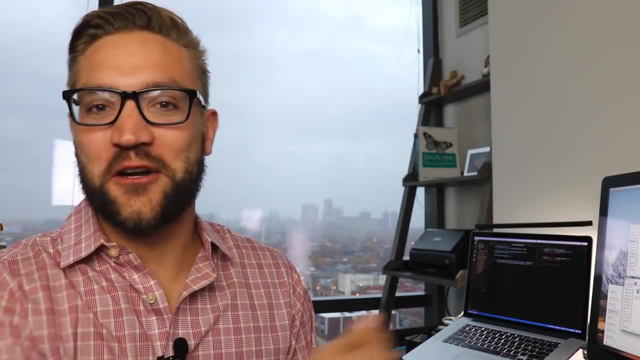 to the code base And in all the organizations that I've been involved with, what happens is when those tests are running, there's a failure. everyone's notified via Slack, so all the developers get a message. you know I'll put in a commit and it fails. And so it's.